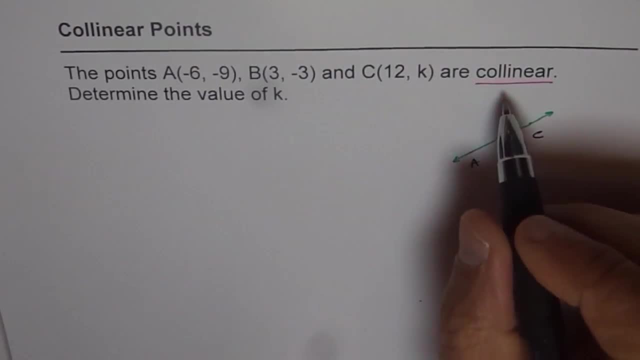 A, B and C here right Now determine the value of K. So point A is given to us as minus 6, minus 9.. Point B is given to us as 3, minus 3.. And C is given to us as 12 and K. So if these three points are collinear, we need to find the value of K. 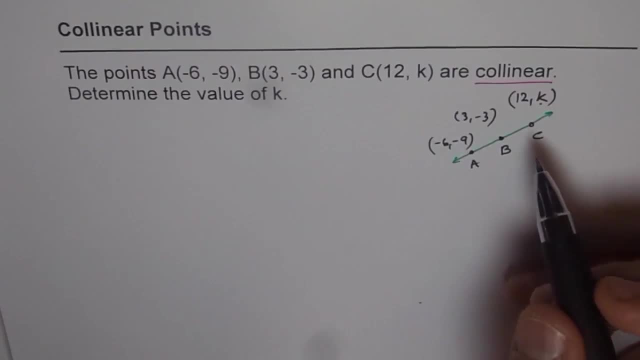 That is the question. So, basically, what we should do here is, using A and B, we will find the equation of a line And in that equation we'll substitute X as 12 and find Y value. That should help us right. So with this strategy, let's start solving this question. So finding 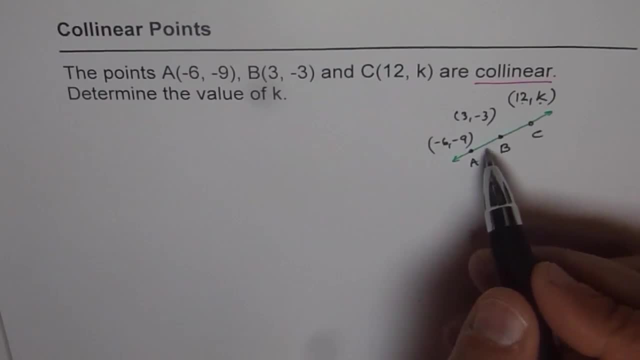 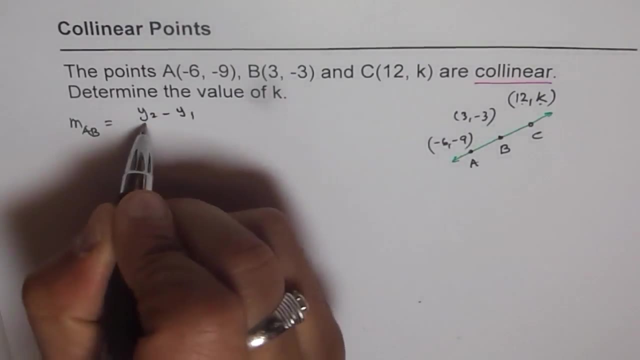 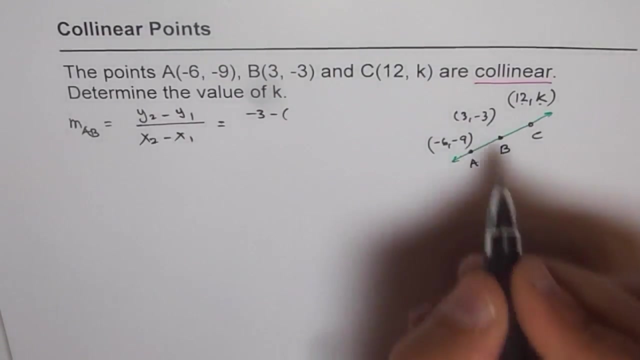 equation of a line given two points That we can do in two steps. First step is find slope between A and B, which is Y2 minus Y1 divided by X2 minus X1.. In this case, Y2 is minus 3, minus Y1 is. 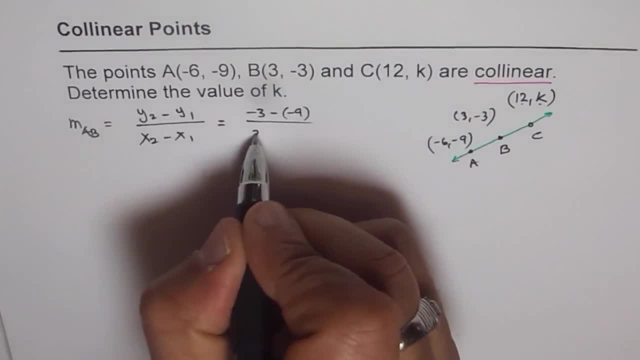 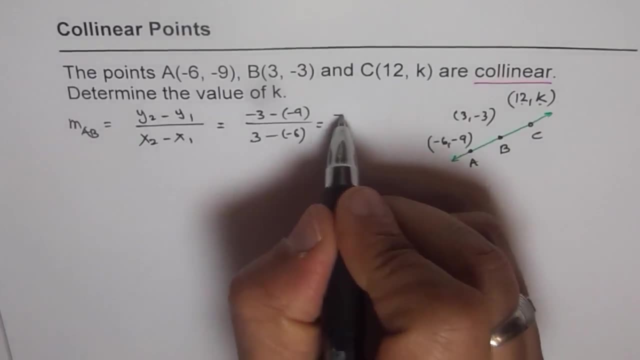 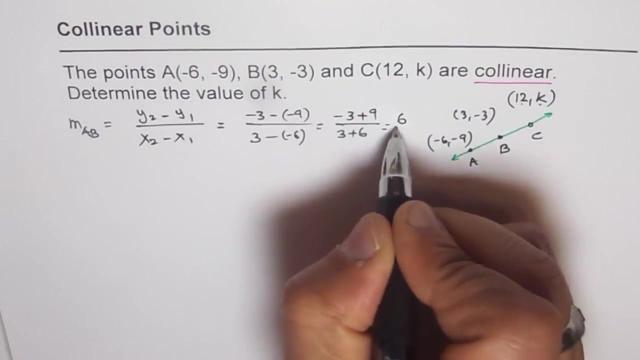 minus 9, over X2 is 3, minus minus 6.. It's good To use these brackets. right Now. let's open these brackets and then solve So: minus 3 plus 9 over 3 plus 6.. That gives us 6 over 9, right, So that becomes the slope. Now we 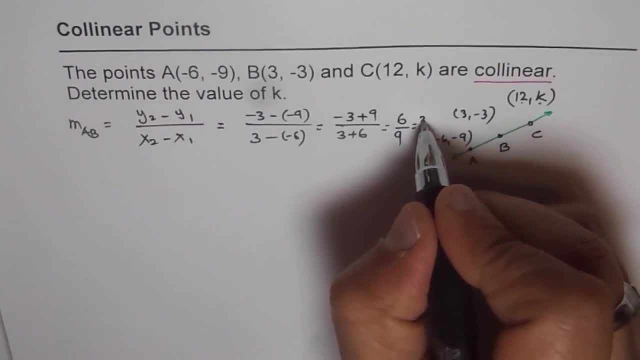 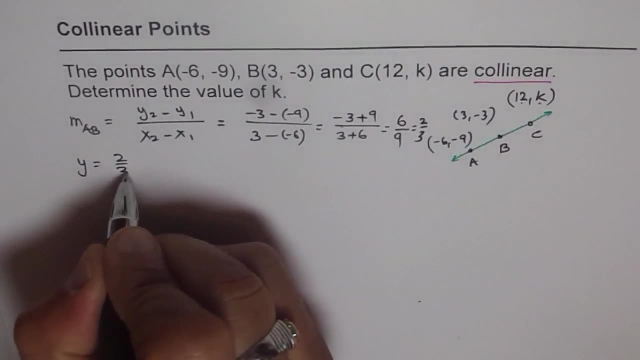 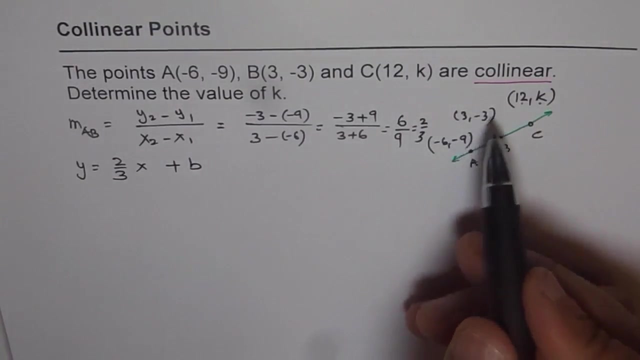 can solve it further, dividing both by 3 to get 2 over 3.. So M is 2 over 3 quarters. Now we can write the equation of a line as Y equals to 2 over 3X plus B. How will you find B? To find B we can use any one of these points. So let's take 3 minus. 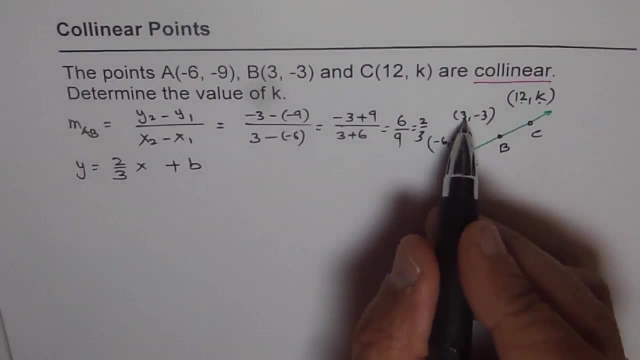 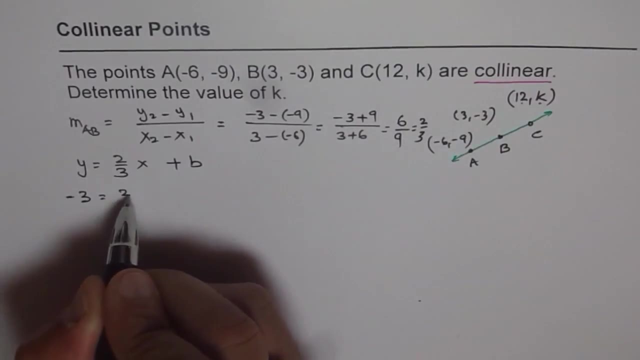 3. It helps because 3 and 3 will cancel out right. So we'll use the point 3 minus 3 in this equation. So minus 3 is Y value, 3 is X value, So we get minus 3 equals to 2 over. 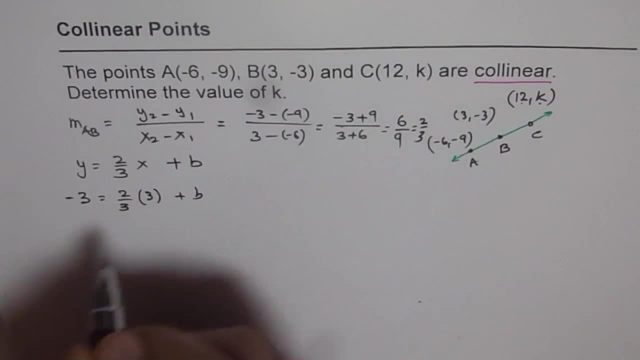 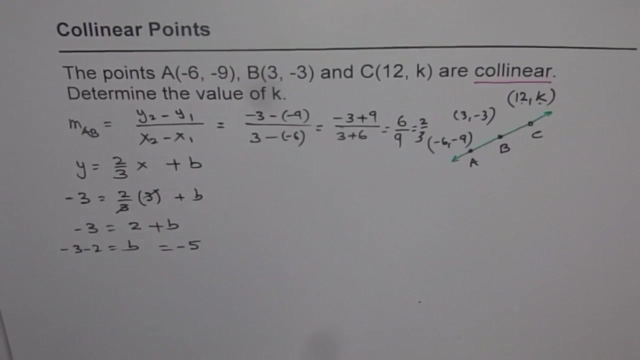 3 and the X value is 3 plus B, So we get minus 3 equals to. this cancels out, you get 2 plus B, And from here you can solve for B. So you get minus 3 minus 2 equals to B, and so B is equals to minus 5, correct. So once you know what, 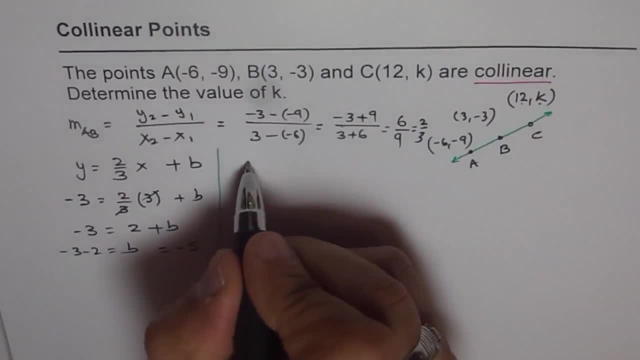 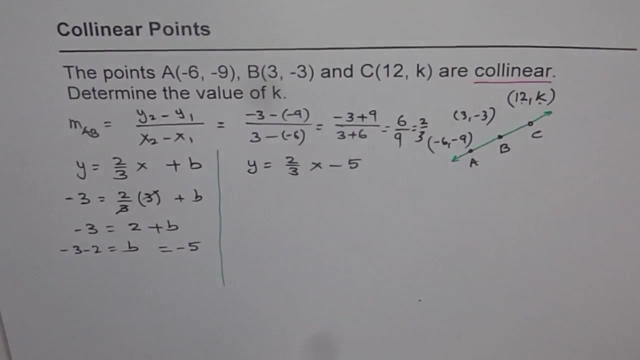 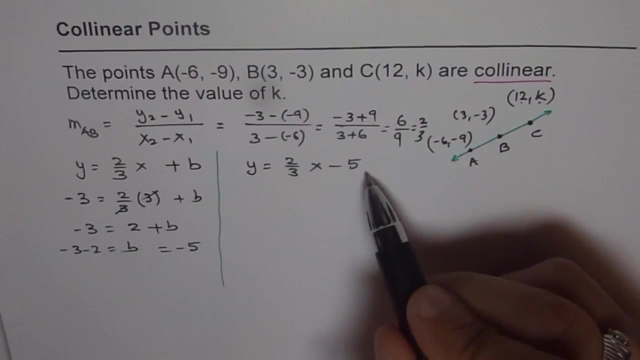 B is, you can write it on your equation. So your equation now becomes: Y equals to 2 over 3X and B is minus 5.. So let minus 5 be. So that is the equation which represents a line through points A and B. Now, if C is collinear, it should be on this line, correct? So we? 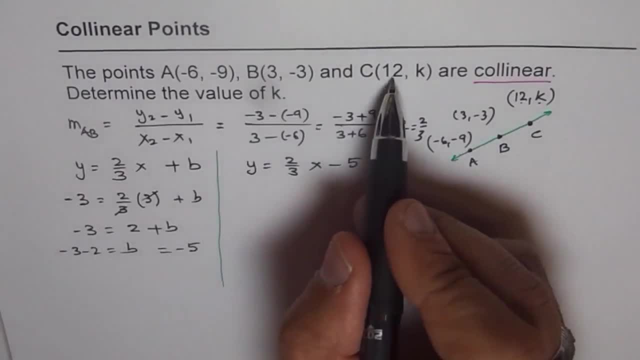 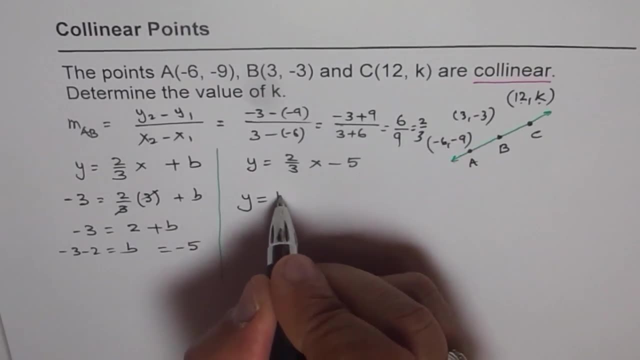 are given X value of C, That is 12.. Subtract 12.. Subtract 12 here and find what Y is. Rather, we could also say Y should be K, So we'll write instead of Y, we'll write K here. now, right? So K equals to 2 over 3 and the X value 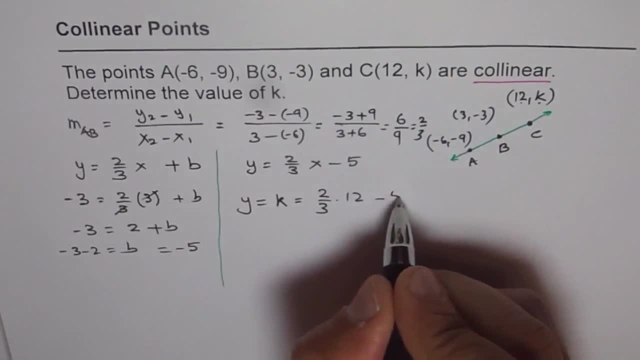 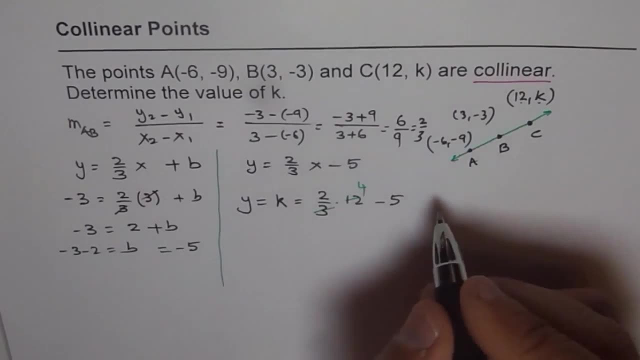 is 12.. So we'll write here: times 12 minus 5.. Now this could be simplified, right? So this goes 4 times, is that okay? So we can write: K is equals to 2 times 4 minus 5.. So 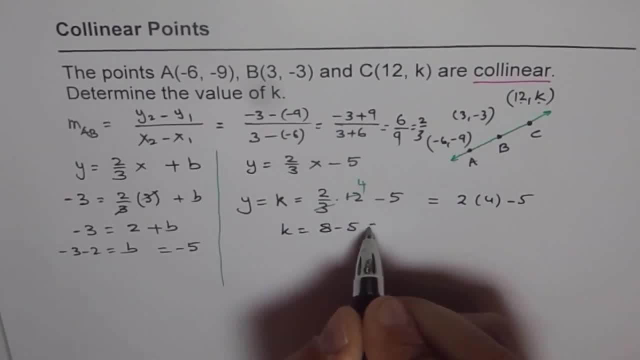 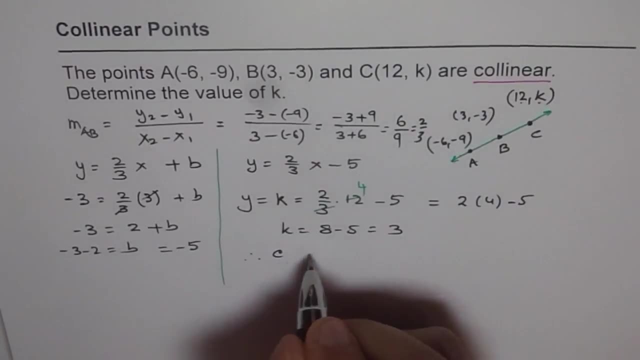 K is equals to 2 times 4 is 8.. 8 minus 5, which is 3 for us. So that is the value of K And therefore we can write down the answer. that is, C should be 12, 3, right? So that should be the point, So the answer. 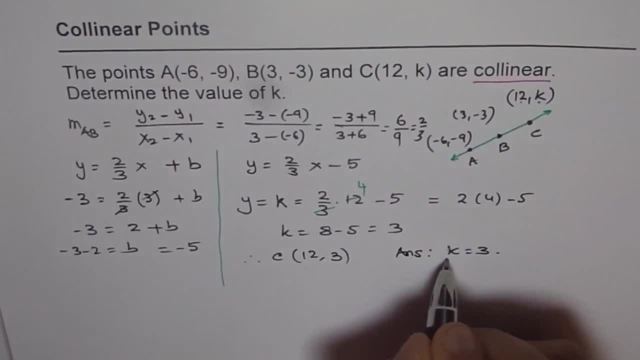 is that K is equals to 3. That will ensure that the point is on the line, and then they are all collinear, right? I hope you understand the method by which we have done it. Let's recap, Let's see what we did here. So first we understand. collinear means that three points. 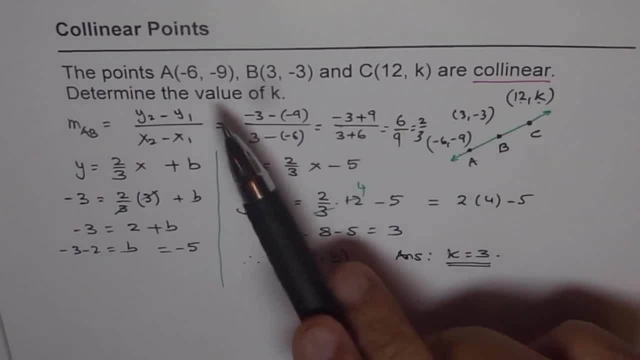 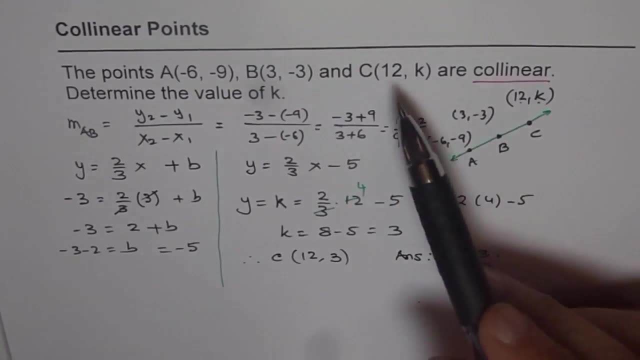 are collinear means that they lie on the same line. Now we are given two points. We can find the equation of a line using the two points. Once you get the equation, you substitute the X value of the third point, find the Y value, which is unknown, K. That becomes the. 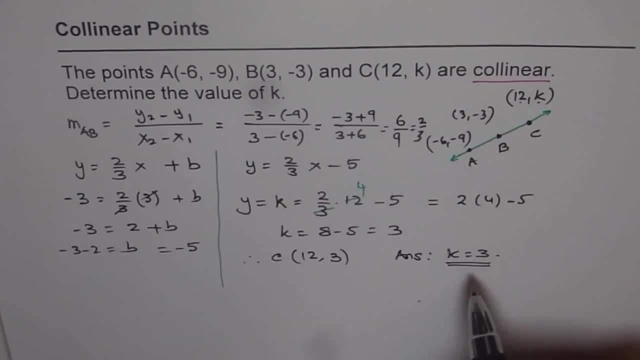 unknown value for us And only for that value of K, that is, only for K equals to 3, this point is collinear. For any other point, any other value of K, this point will not be collinear, It'll be. 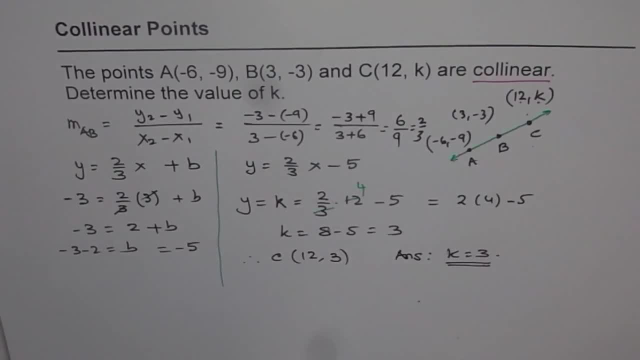 not on the line, but somewhere else. I hope that's absolutely clear to you, right? Thank you.